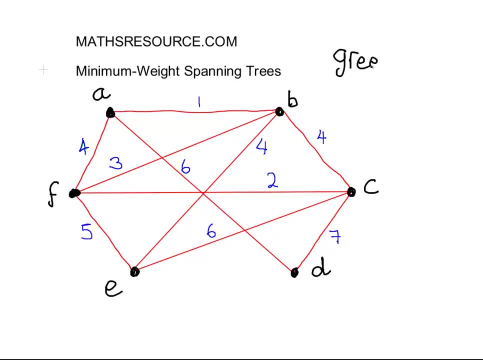 Let's just write that Greedy algorithm. So what we're going to do is continually select an edge, having minimum weight, But each time we have to avoid making a cycle. Now, I'll sort of come to that shortly, when the time comes. 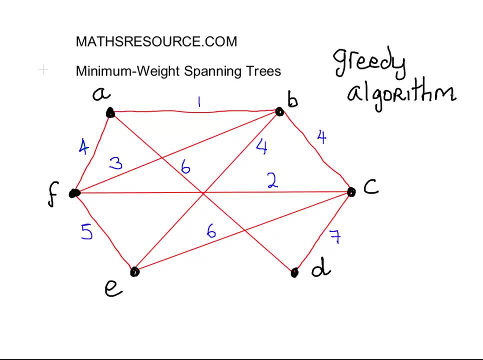 So, just as a remark, actually, what is the weights of each, Each edge? Well, AB here is 1.. Let's just write that in again. BC there is 4. C to D is the weight of that edge is 7.. 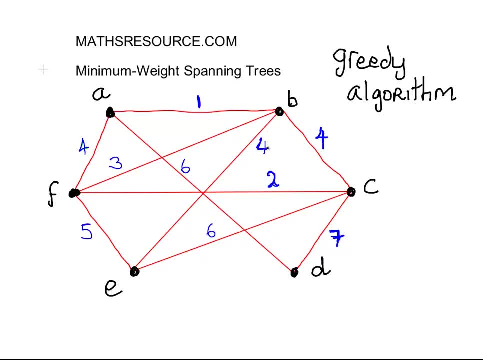 C to F is 2.. That's a small one. B to E is 4.. C to E, that's 6.. A to D: A to D is this one here, that's 6 as well. B to E is this one here, that's 6 as well. 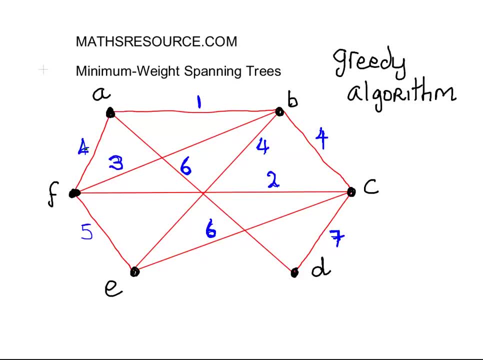 B to E is this one here, that's 6 as well. B to F is 3,, A to F is 4, and E to F is 5.. So those are all our edges Now. pretty clearly, you can tell that the minimum edges. 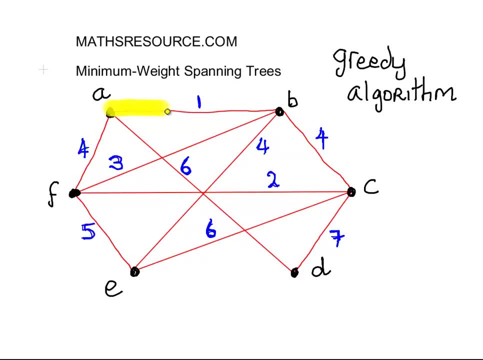 the edges with the lowest weights are the first two. just to start off with are A and B. and also well, A and B is the first one, So that's the first one picked, So I'm moving on to the second one. 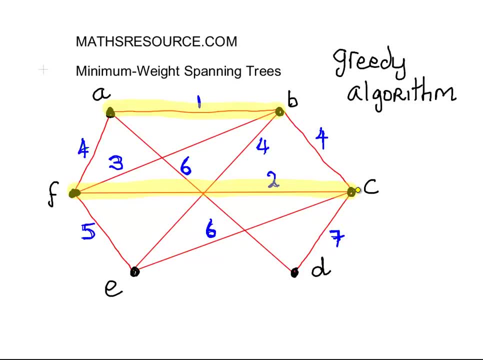 Almost immediately, And that's C and F. Okay, So the next one I'm going to pick is the next shortest one after that. So I'm going to put a little circle around all the ones I've picked Just to sort of indicate that they're out of action. 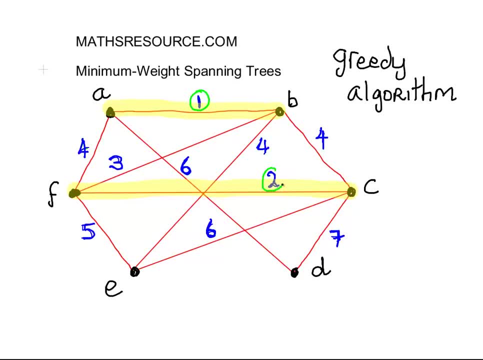 So that one's gone. This one here is gone. The next shortest one after that is B to F. Okay, So let's pick that one there. Okay, So that one there is picked. Okay, Now, this is what we have so far. 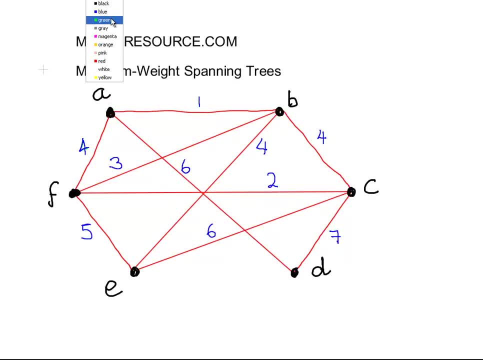 I'm just going to move on to the next slide And I'm just going to sort of pick out what we have chosen so far. So we have picked this one out first, That one there. We put this one out second Because it's two. 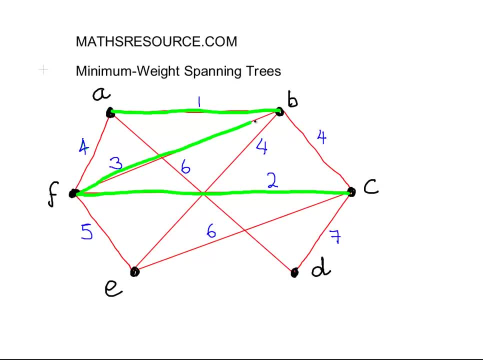 And we picked this one out. third, because it has a weight of three. So far, so good, But what we've got to worry about now is where do we go with the next one? So what's the next smallest weighting? We have a couple of fours knocking around. 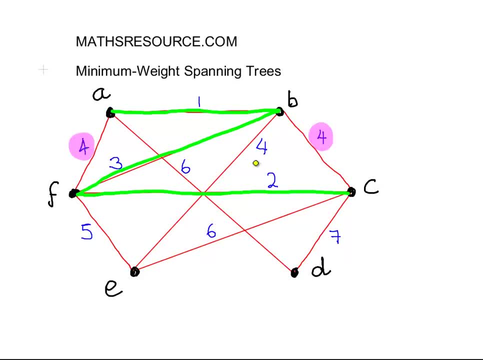 We have a four here, We have a four here And we have a four here. Now, the thing about this, This four, this one here, is that if we pick that edge, that's the edge A to F, we're getting a cycle: A, B and F. 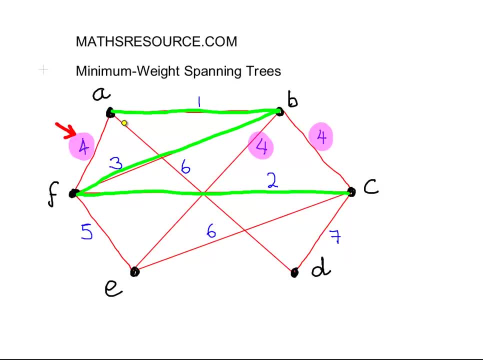 So if we pick that edge there, we're getting this cycle here. I'm just going to draw it in quickly. That's a cycle. That's what we don't want. That is not a minimum spanning tree, So we can't pick that one. 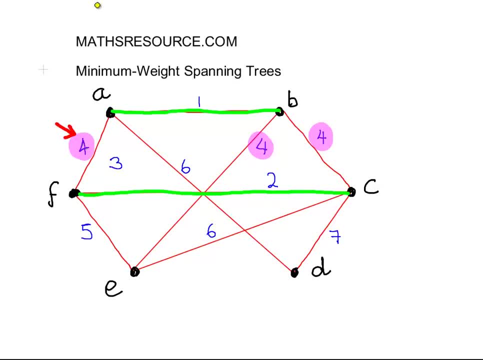 Likewise. I've just taken out one of my edges there, Sorry. Likewise, we can't pick the one on the right-hand side, because if we pick that one we also get a tree, So just put that one back in there. So if we pick B, C, we're getting a cycle A, B and F. 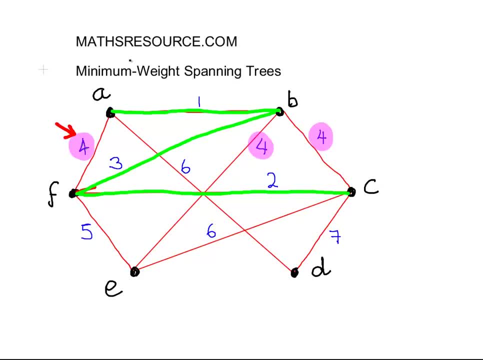 So the one we have to go for is B2. And E, So let's pick that one there. Okay, So this is the one. we've selected this one here, because if we pick any of the other two, we would get a cycle. 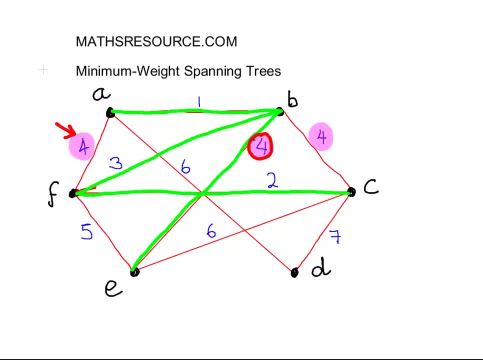 And a tree does not have cycles, So we're picking that one there. Okay, So let's just sort of cross off the ones we have picked already. We can't pick that one because that will give us a cycle. We can't pick that one because that will give us a cycle. 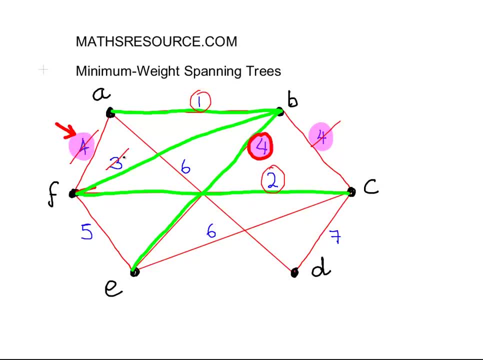 We have picked this one already. We have picked this one already And we've picked that three already, So the next thing we can do is that could be The next smallest weighting. there is five down here. The thing about that one is, if we pick that five, 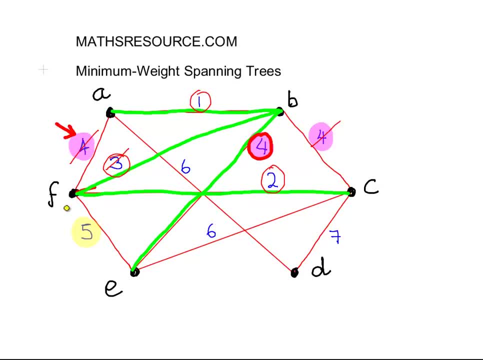 we're getting a cycle between. We're getting a cycle So we can't pick that one, So we're going to cross, So we're going to cross that one off our list And we're not going to pick that. What do we have to do exactly? 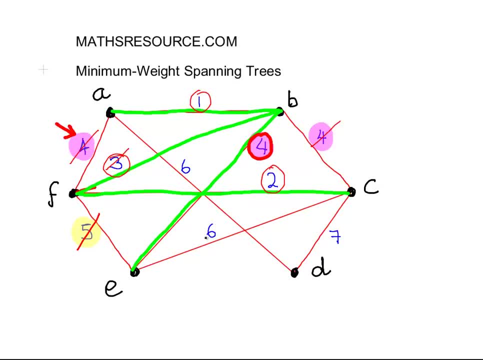 What's our final destination. So the last thing we have to do is actually just remember what we have to do. So we have to connect each vertex of each of the vertices, But there's only one left, anyway, Okay. So What do we do now? 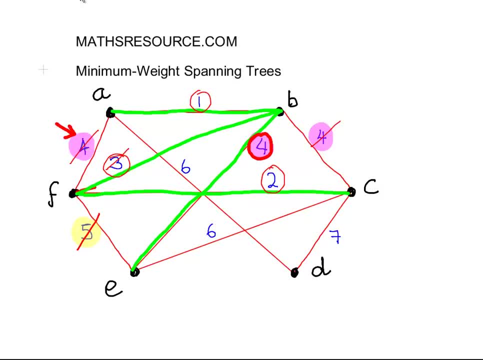 So actually just think about this: We either pick this edge here- I'm just going to make it a bit thicker- This edge here- C to D, That will complete the spanning tree Okay, But E to D would actually give us a smaller spanning. 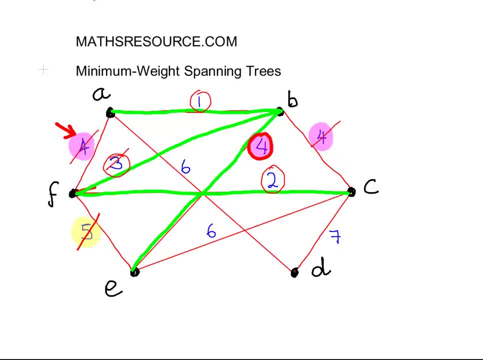 Or a spanning tree with smaller weighting. So what we're going to do is pick E to D instead. Okay, So that's done. All our edges, all our vertices are connected. Okay, And so, therefore, we now have a minimum spanning tree. 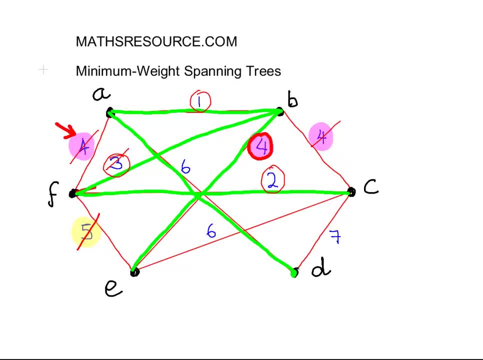 So, just as a remark, we have six vertices, So we should have five edges. Now I could have sort of just made that remark there earlier. So we picked this one first. Oops, We picked this one first, This one second, This one third. 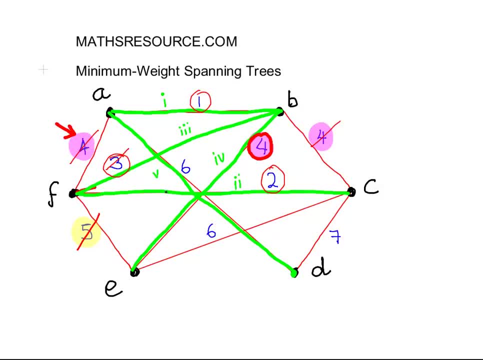 And this one fourth, And this is our last one here, The fifth one here. Okay, So we have all our edges anyway. There's only six vertices, So there's only five edges that we were looking for, And there's no cycles.